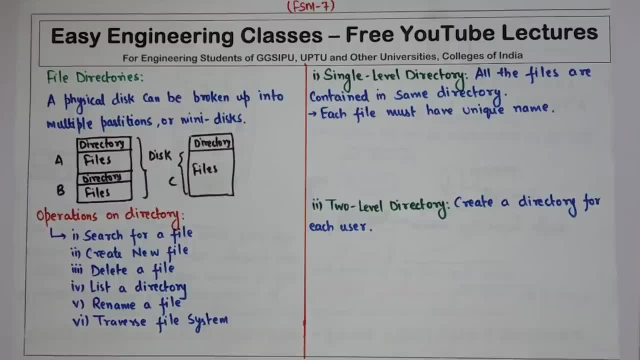 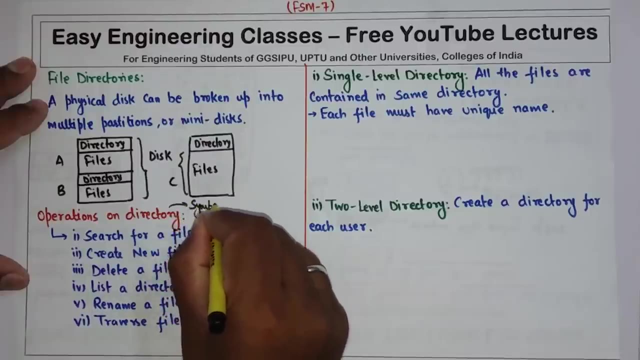 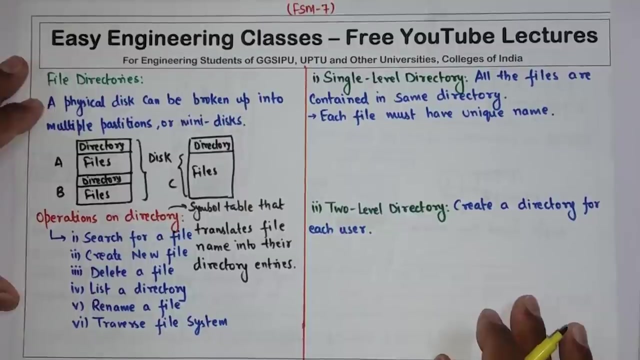 a directory is. so a directory can be viewed as a symbol table that translates file name into its directory entries. so directory is directory is a symbol table that translates file names into their directory entries. now you can think of this as a phone directory, where you have the details of each of the contact. similarly, there is a directory file directory. 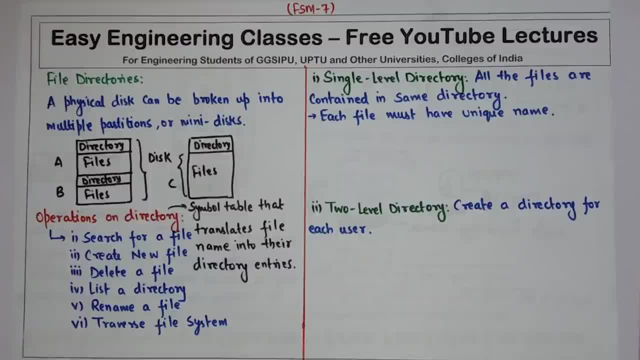 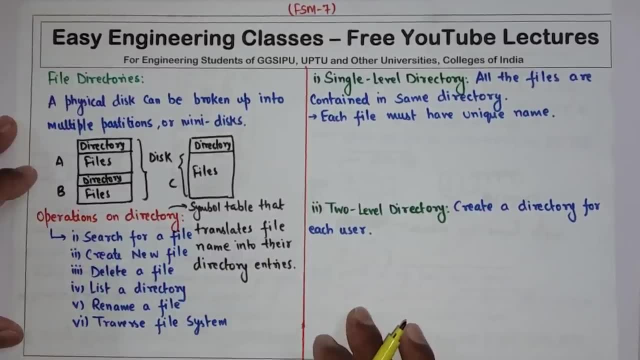 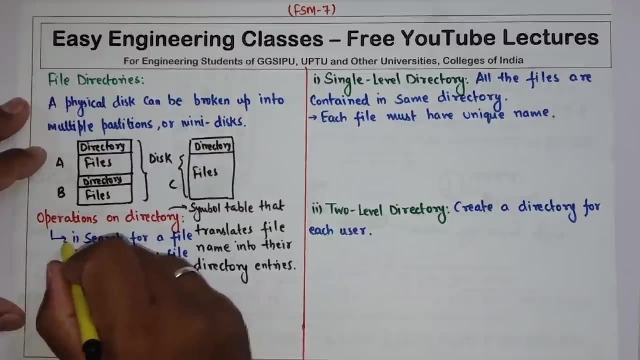 that contains the information of each of the file in your operating system. now, as you can do different operations on a phone directory, similarly, in a similar way you can have different operations on file directory also. so first you can search for a file in the file directory, then you can create new file inside a directory. delete a file, list a directory, rename. 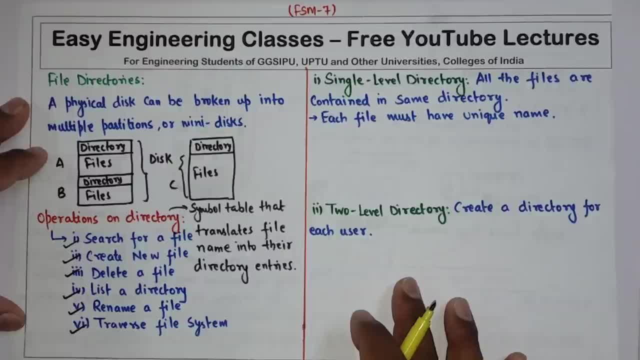 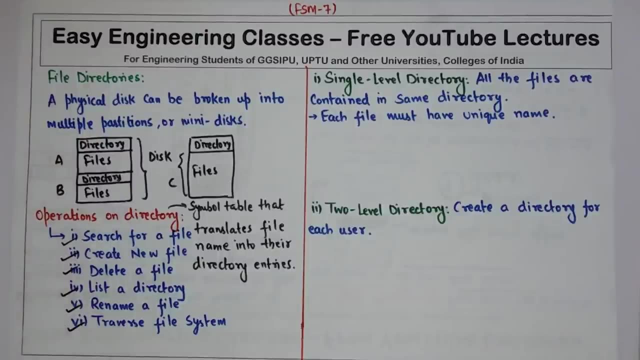 a file and traverse entire file system. so these are different operations. these are self-explanatory, so i am not going into the detail of this. the important point for this lecture is there are different schemes of the file directory system in an operating system and we are going to see. 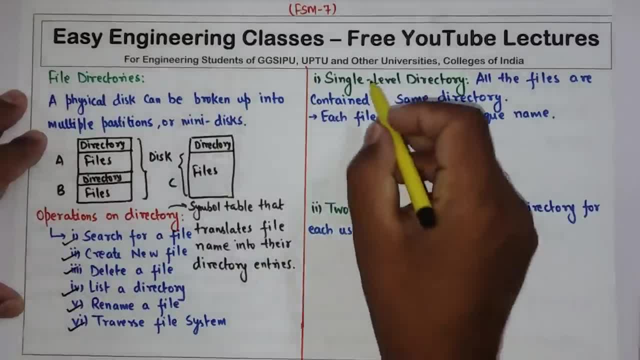 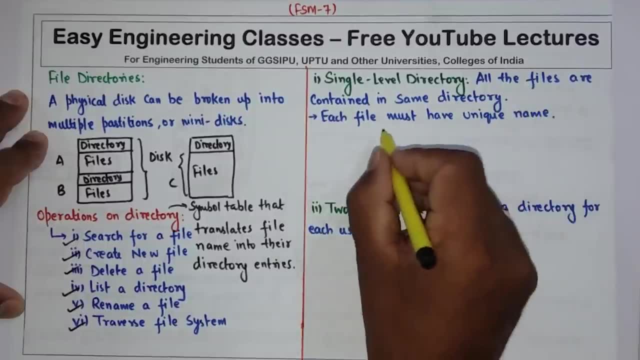 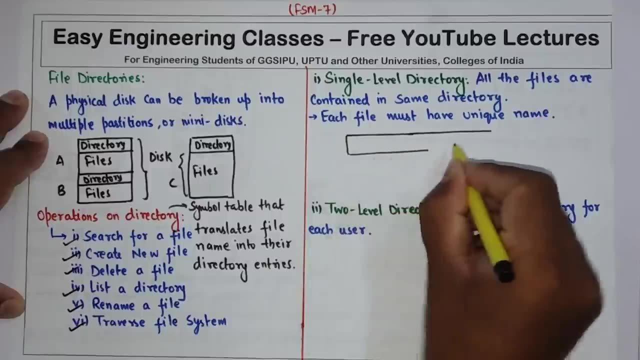 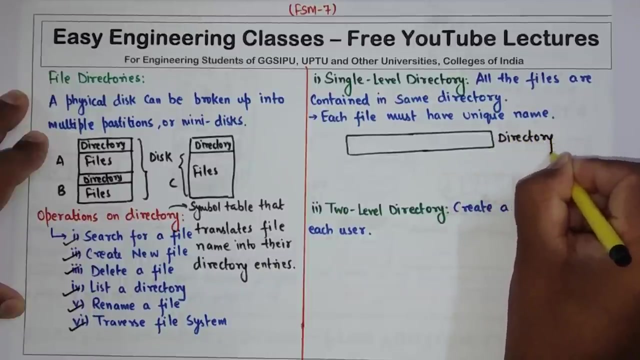 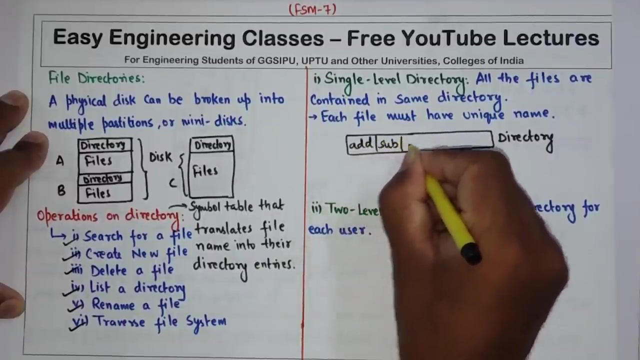 those different schemes. the first one is single directory or single level directory. in this all the files are contained in the same directory. so let's say, if i have a directory like this, this is the directory. this directory is at the same level and inside this directory you can have different entries like addition, subtraction, multiplication. 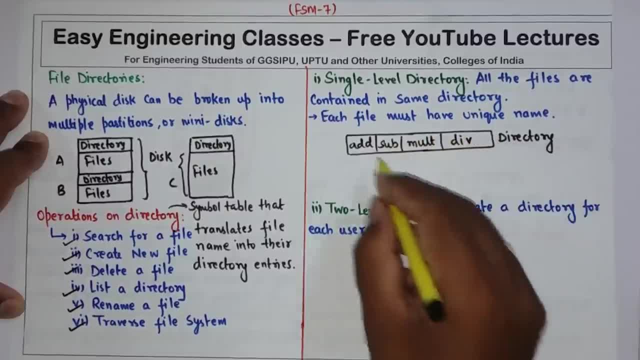 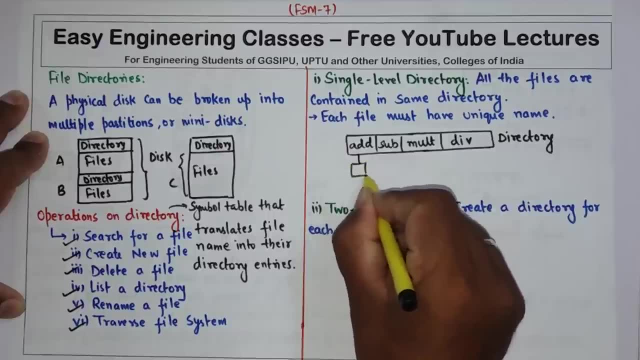 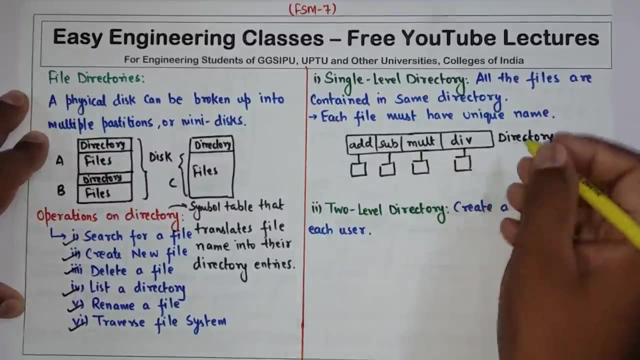 and so on. suppose i have this, five different entries and inside this you can have your files. now, as you can see that all the files are at the same level inside the same directory, so the file must be have, must have unique name. say, if i have a file of this as f1, i cannot have this as f1. this 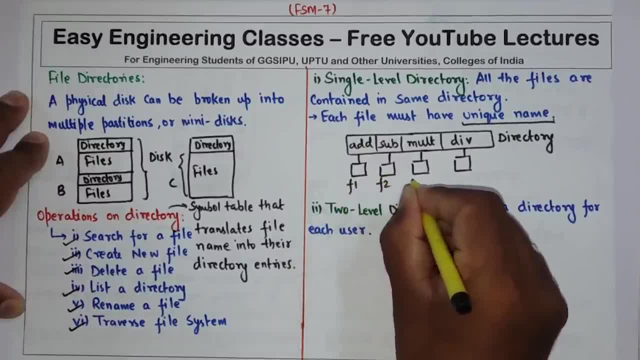 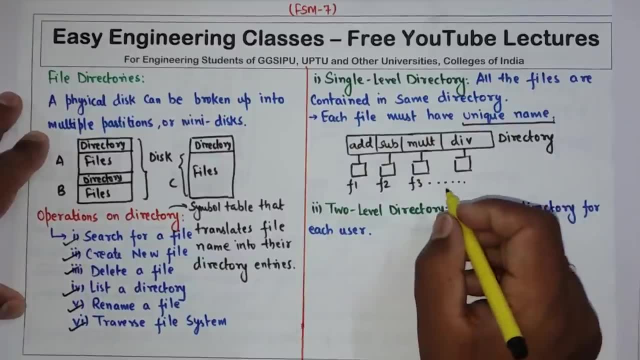 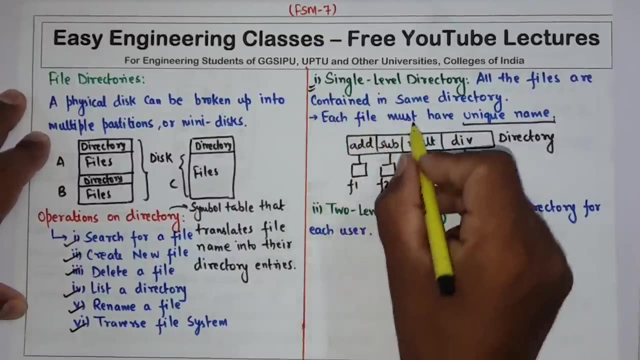 has to be f2, f3 and so on. if i have two files with the same in inside the same directory, then there will be some ambiguity in calling the file names. so let's see how it works. so in single level directory you have to have a unique file name. 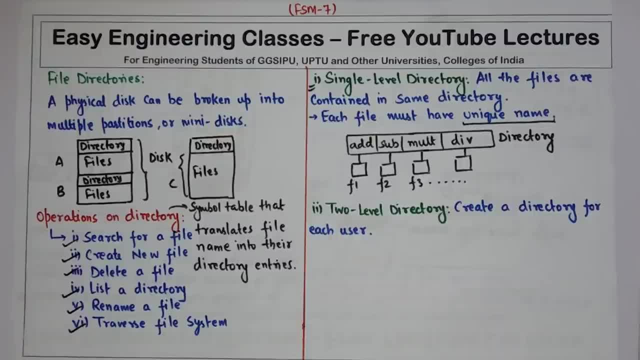 but the problem with single level directory is that if there are lot and lots of files, the names for those files needs to be unique and that is a tedious task to look for a new name every time you create a new file. so to overcome this, that disadvantage, there is two level. 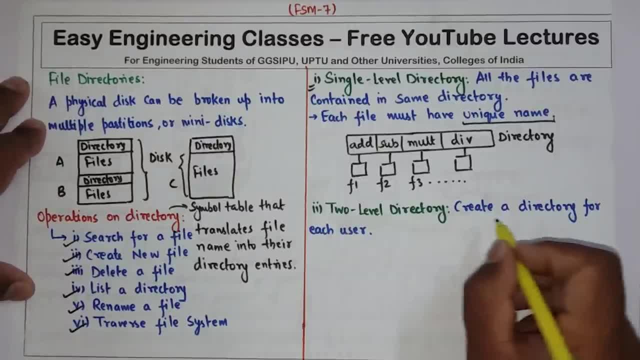 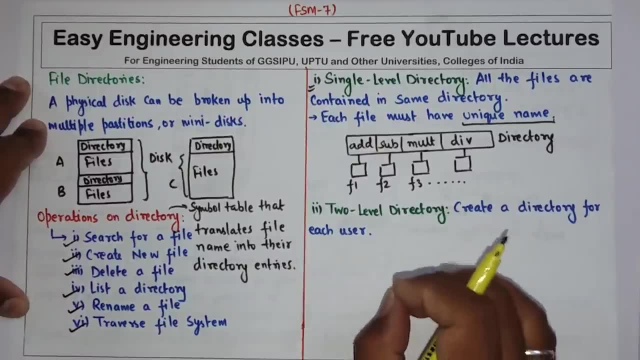 directory system. now the two level directory system says: if there are 10 users in an operating system, then create 10 directories for each user or 10 directories for 10 user. that means one directory per user. so if i have a three user system in my system, three users in my system say user one. 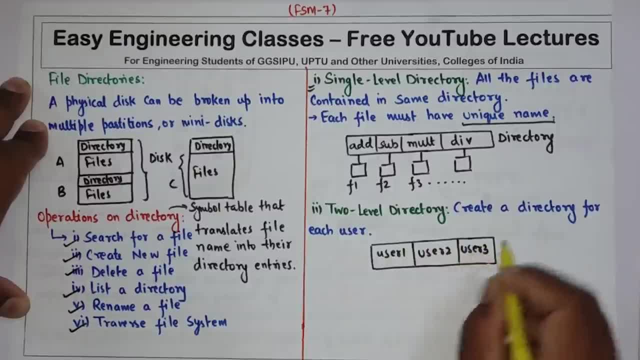 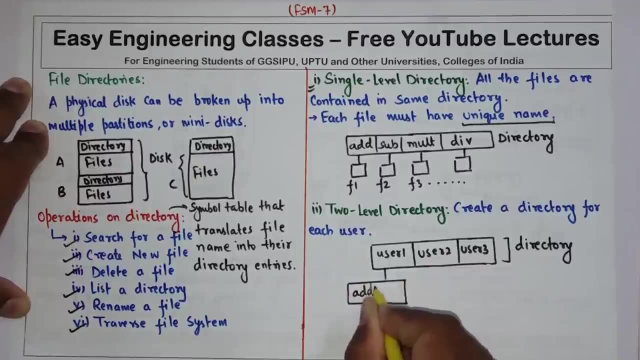 user two and user three. so this is first directory or directory level one, and for each of this user i can have different directory, similarly for user 2 and user 3. so this is two level directory system and now inside this i can have my files. so create a directory for each user is your two level directory system. 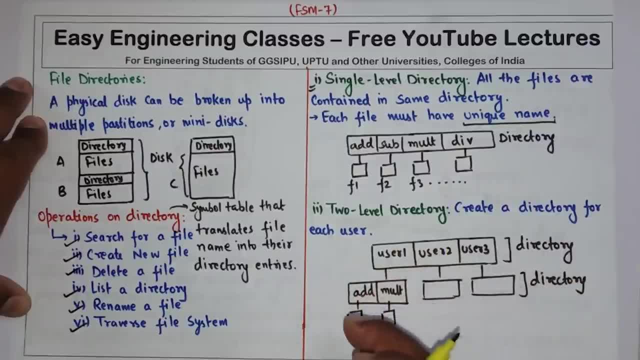 now, in this you don't have to worry much about the uniqueness of the file name because a single user has its own directory. so if this is file for f user 2 and this is file for user 1, this can have f1 file name and this can also have f1 file name, but inside the same directory inside. 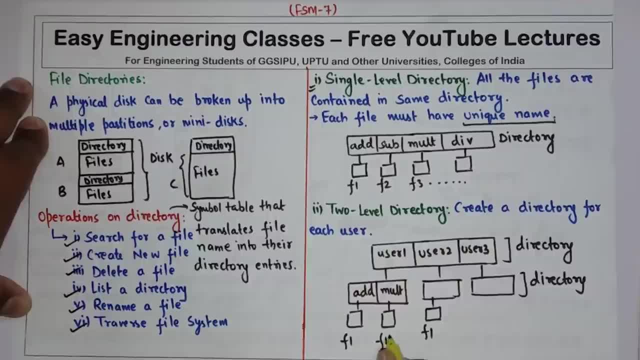 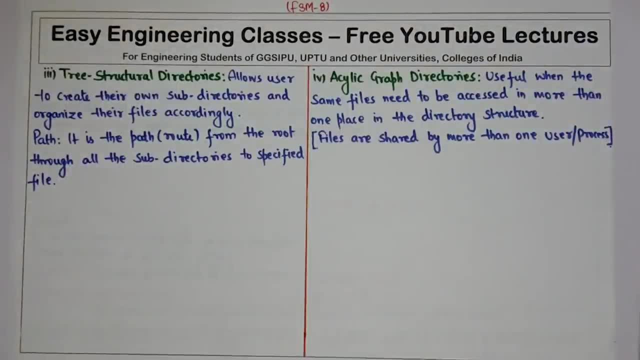 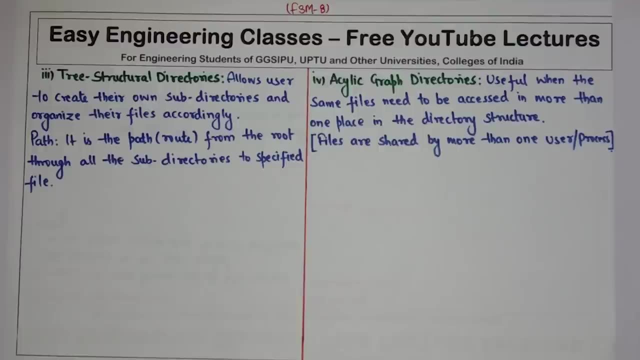 the same user, file name should be unique. that means it cannot have f1. so that is clear. that is two level directory system. next is the extension of the two level directory, which is tree structure directories. it allows the user to create their own sub directories and organize the files accordingly. 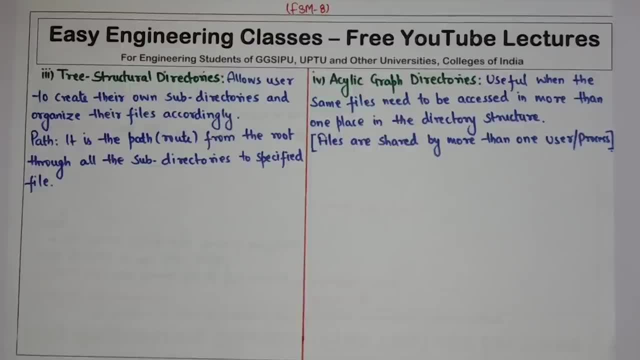 now, like any tree in data structure, there is a path. what is a path? path is the root from sub directories, so or alone, and the path is only path. so which is this? cores thru theirapo, transitioning user in service and container system and other 1ly names publicly is functionally знаем. 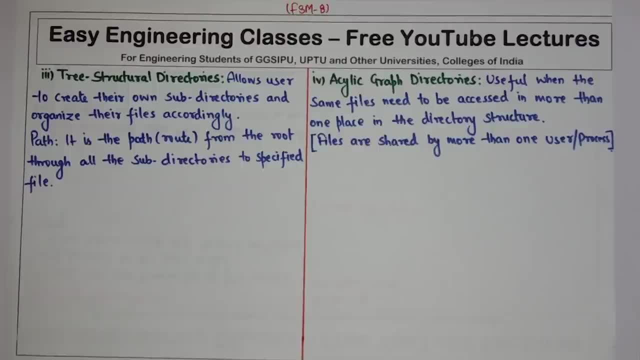 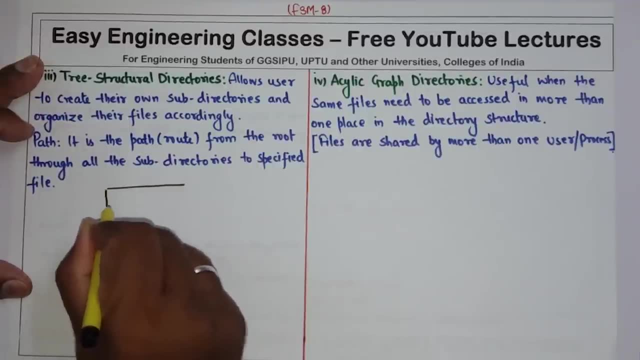 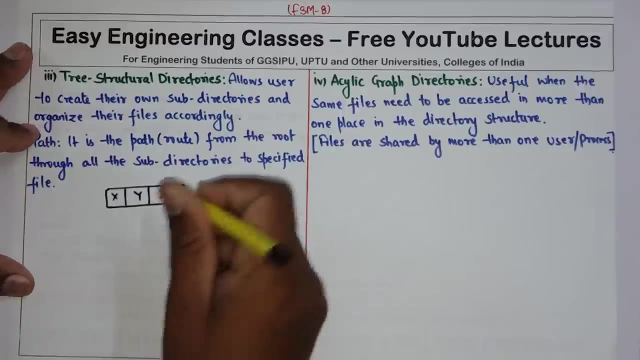 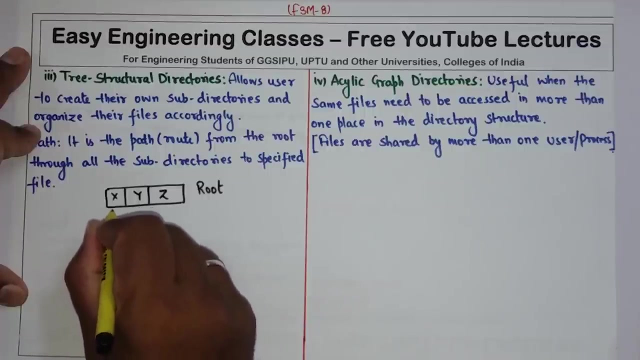 the root node through all the sub directories to a specified file. so for example, if I have a tree like directory, like this, on top I should have a root, say X, Y and Z. there are three directories on that root. now in this each user can have its own directory system. so for example, X can have a. 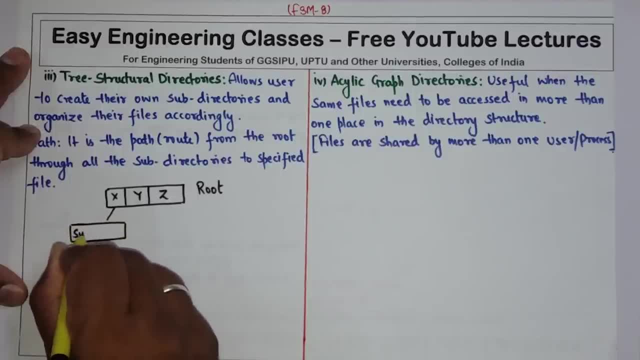 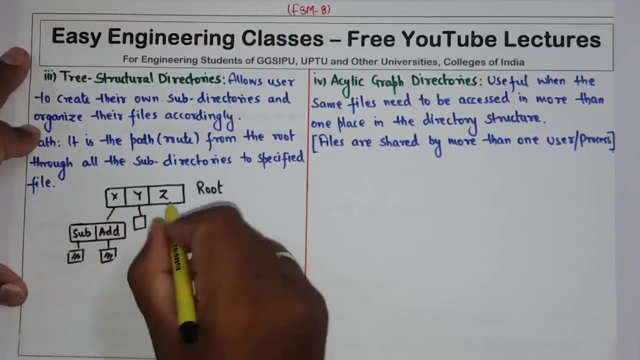 directory like this, say subtract add and can have files inside these directories and Y can have files directly, no sub directories and Z can have more level of directories. so for example, Z can have something like this: math and English, and inside math Z can have subtract addition and the files. similarly in English Z can 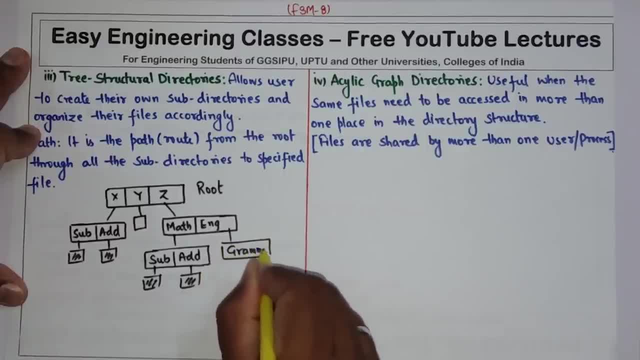 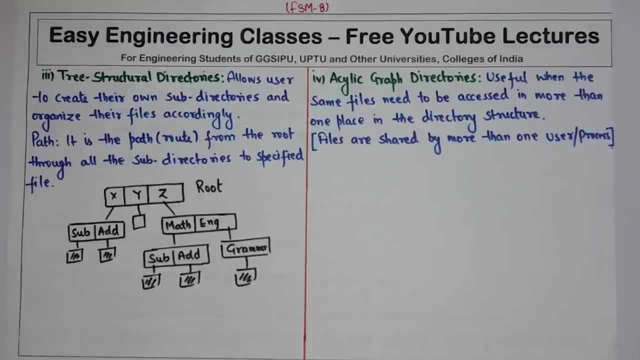 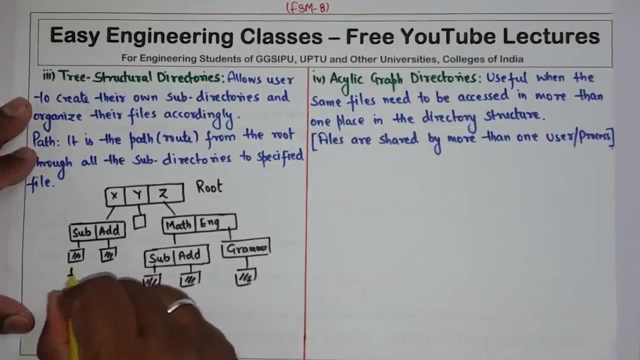 have grammar and files. so in this way, the users are creating their own sub directories, managing the files as per their need. that is your tree structure directories. now what happens if more than one users wants to share files like these files? this file, say, suppose F1 and F2, this can also be F1 and F2. these files are same. 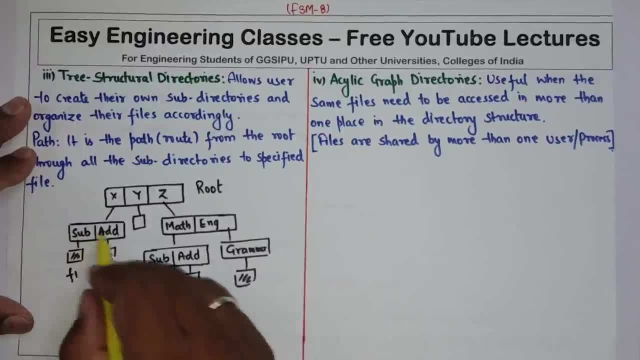 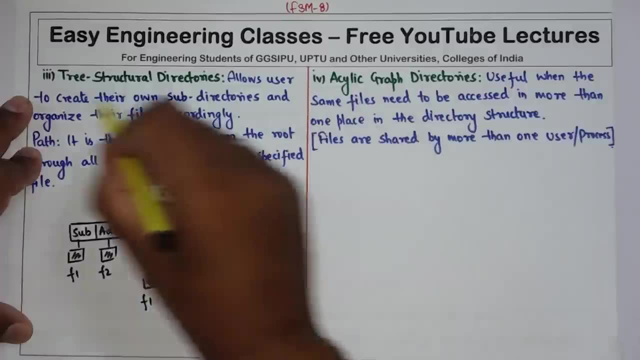 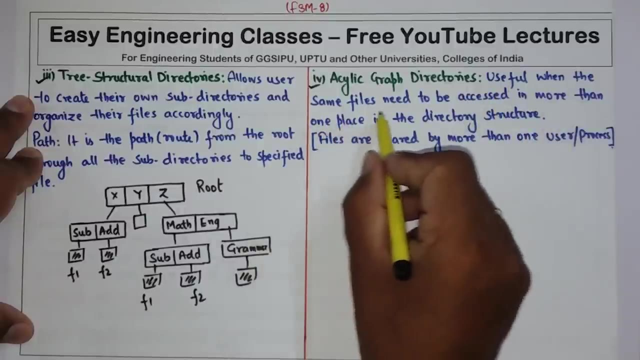 because they are under same sub, subtraction and addition, so they may be a chance that X and Z wants to share these files, so that provides the concept of acyclic graph directories. it is useful so in order to share files with a user. It is useful when same files needs to be accessed in more than one place in the directory structure.